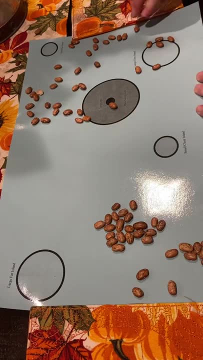 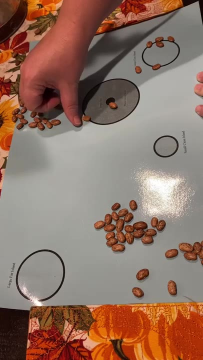 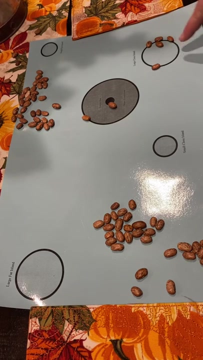 These have not landed on anything. Okay, these guys over here have not landed on anything. Okay, this guy wasn't, This guy didn't. That guy's on a line, so he's good. This guy didn't, So this one has one, two, three, four, five species that landed on the large close island, two on the main ecosystem, So we're going to repeat this process for a total of five dispersal events. 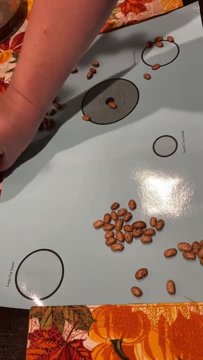 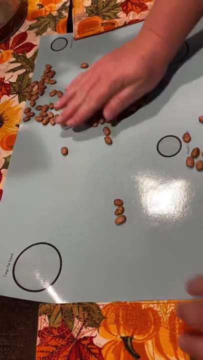 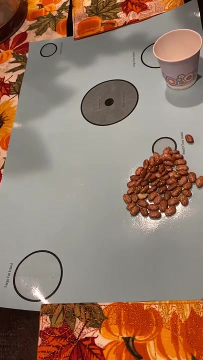 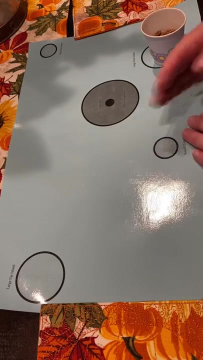 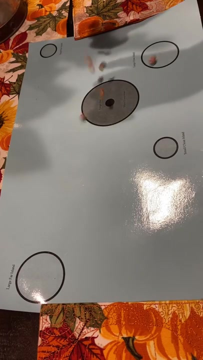 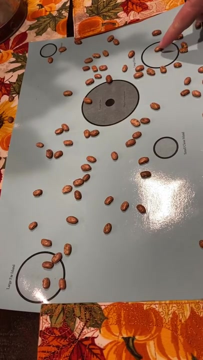 Okay, so I'm going to collect all my pinto beans. Get them all together now. Okay, collect them all And we'll do another dispersal event. Here is dispersal event number two. Okay, there's dispersal event number two. We have one on the large close island, two on the main ecosystem, but this time we have one, two, three, four on the large far island. 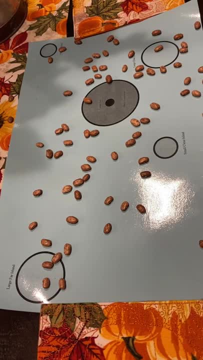 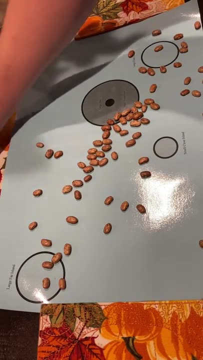 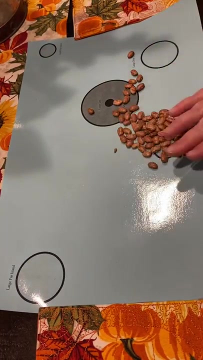 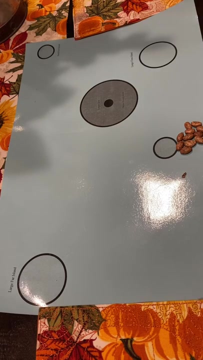 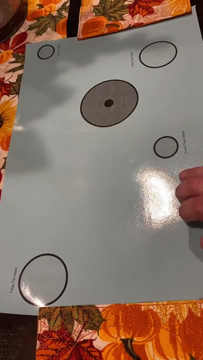 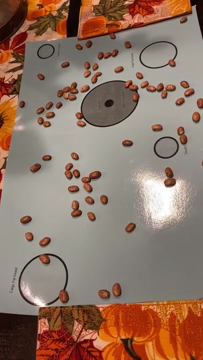 So that is dispersal event number two. Let's collect all of our beans. They kind of go everywhere. Get ready to do dispersal event number three. Hold that back down. Here we go with dispersal event number three. Okay, dispersal event number three. 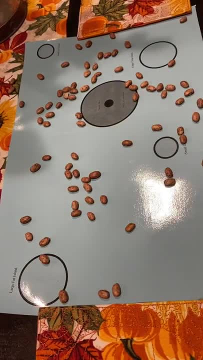 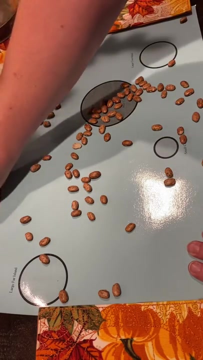 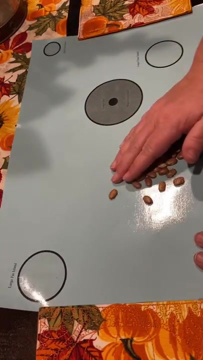 That is not on the line. So we have two on the far large island, one, two, three, four on the main island. So that is dispersal event number three. Let's collect all of the beans again. Now we're going to get ready for dispersal event number four.